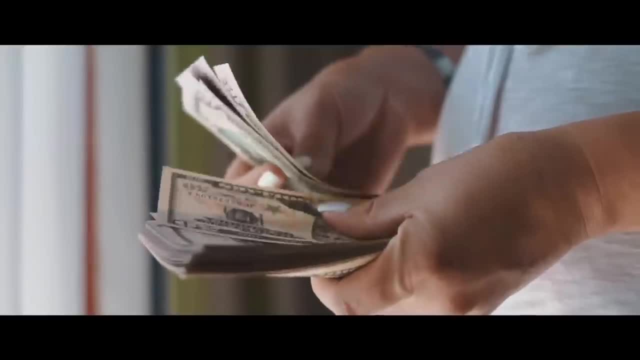 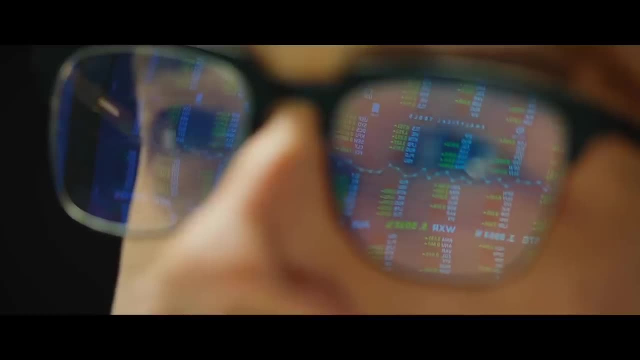 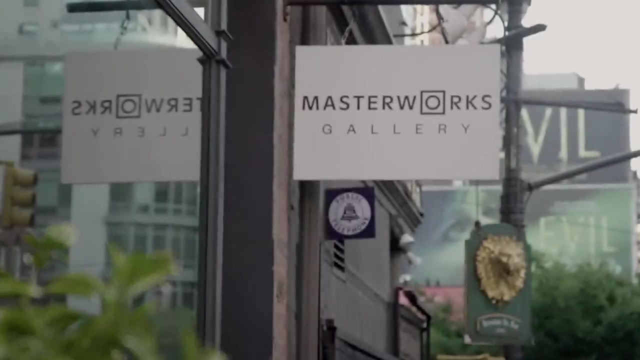 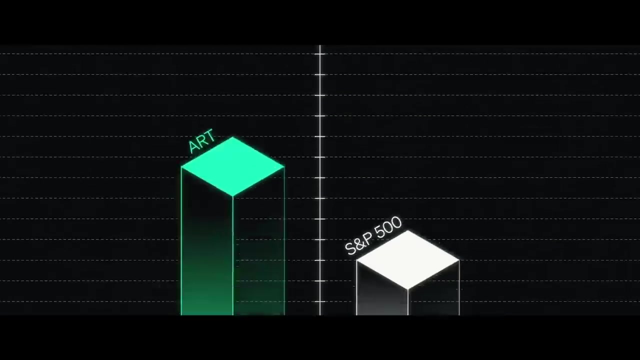 video Masterworks. Masterworks is an award-winning startup in New York City that allows people like you and I to invest in blue-chip art. Traditional assets can lose value due to current events, but the value of art may not be as subject to these conditions. You could value an original Picasso painting. 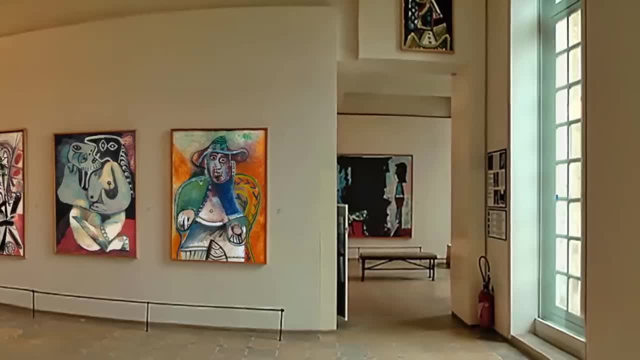 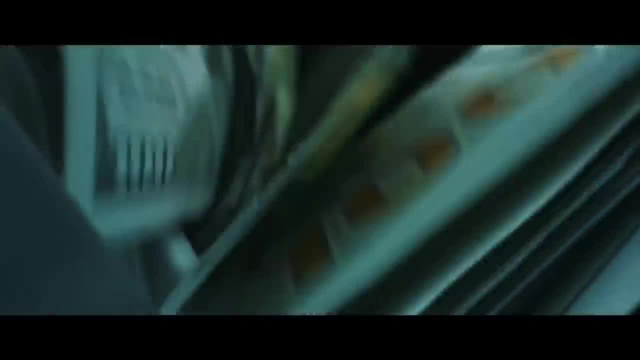 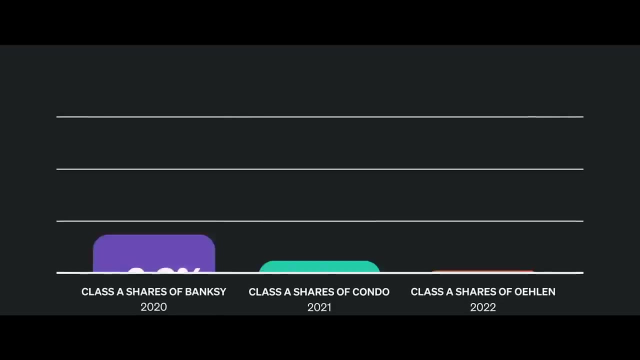 anywhere right now, and even with the current economic state of the world, you'll still retain its value. With countries currently dealing with record high levels of inflation, this is now especially important. The last time inflation was this high. art appreciated at an average of 17.5% per year, according to the Masterworks All Art Index. 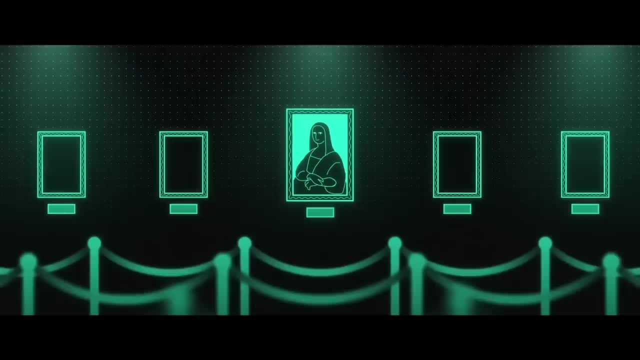 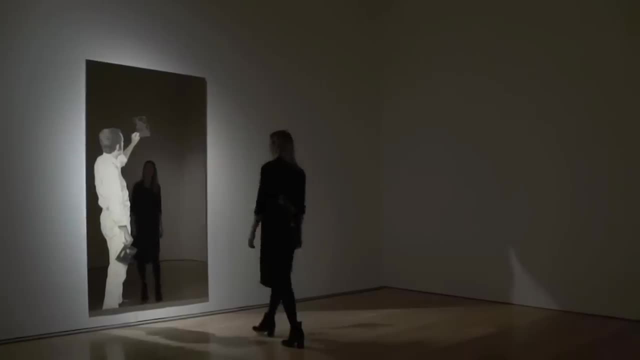 which was almost double the rate of inflation in the same period. Masterworks gives you the potential to see returns on artwork from world-renowned artists. This isn't The Metaverse or NFTs. this is tangible contemporary art from established artists with track records of high. 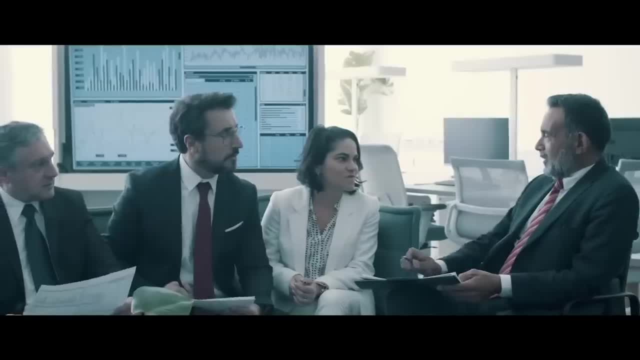 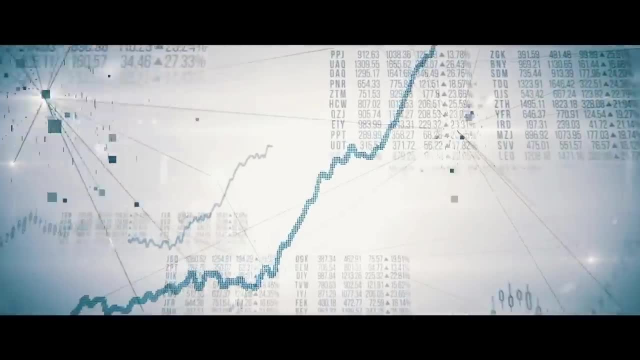 value works that sell for hundreds of thousands, And the results speak for itself. In eight of their nine exits, Masterworks has delivered net returns over 13.9% to their investors. Shares of paintings by artists like Banksy, Kaws and Basquiat have sold out within minutes. 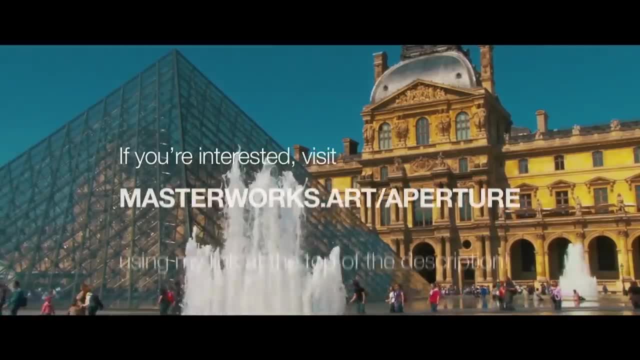 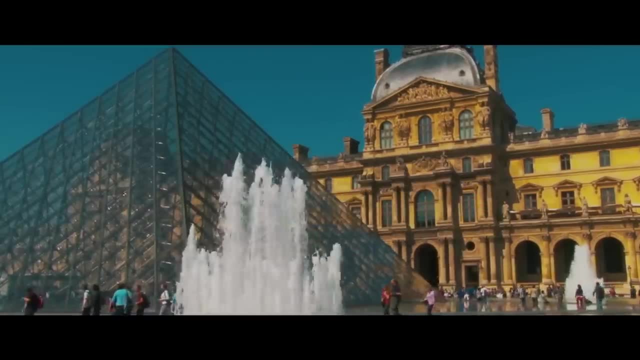 It's easy to see why demand is growing, but subscribers can skip the waitlist today with the special link in the description. Net return refers to the annualized internal rate of return, net of all fees and costs, calculated from the offer and closing date to the date the sale is. 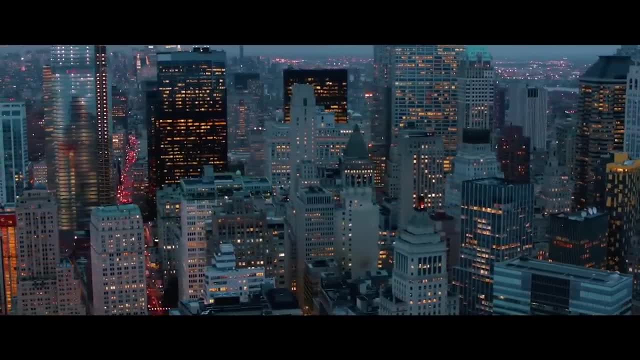 consummated. This means that you'll be able to sell your artwork at any time, regardless of the price. IRR may not be indicative of Masterworks paintings not yet sold and past performance is not indicative of future results. See important reggae disclosures at masterworkscom. slash cd. 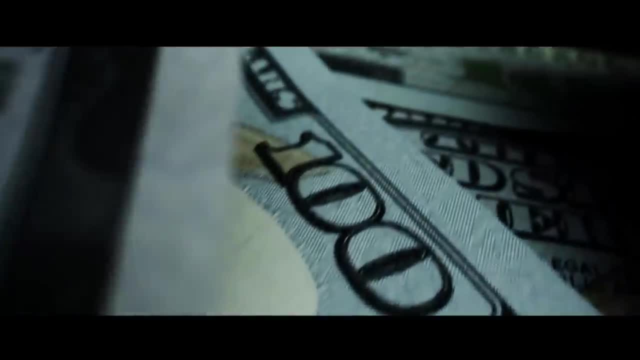 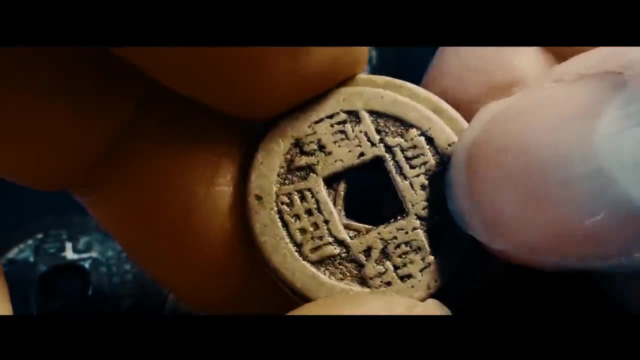 Back to our story. Contrary to what you might think, money as we know it today, at least in its physical form, has remained largely unchanged for millennia. The first sign of what we might think of as a banknote took the form of a piece of leather. 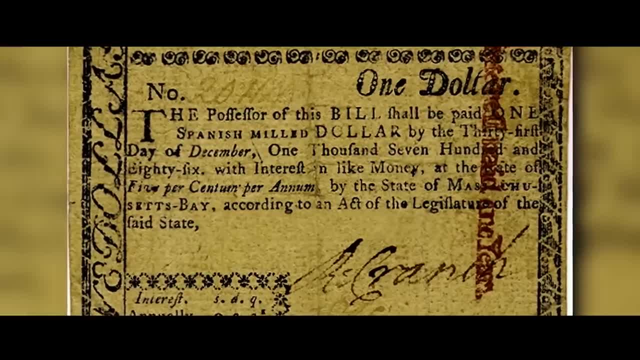 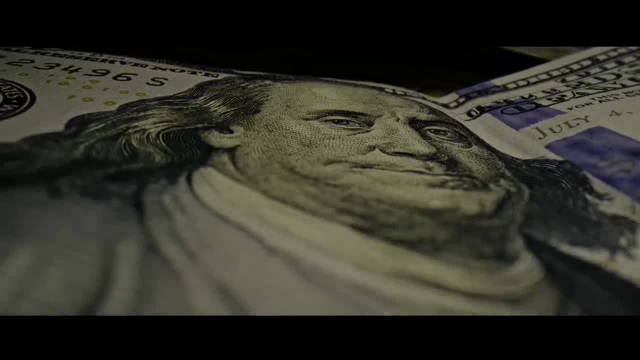 in China in 118 BCE, and 900 years later, paper currency came to fruition. It would be another several hundred years before this kind of currency would make its way to Europe and then the rest of the world. Centuries have now passed, yet the basic concepts invented by 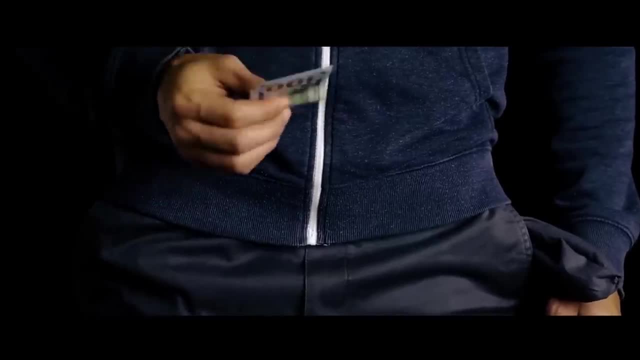 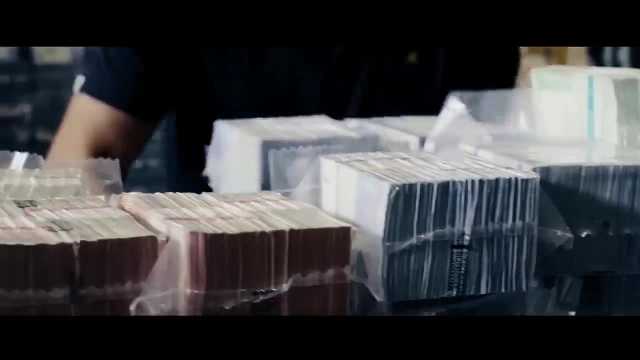 the Chinese aren't that distinguishable from what we have today. In fact, the only real difference is what these notes and coins represent. The first real global system of value in currency was the gold standard, which began in England in the early 1800s. It tied a currency's value. 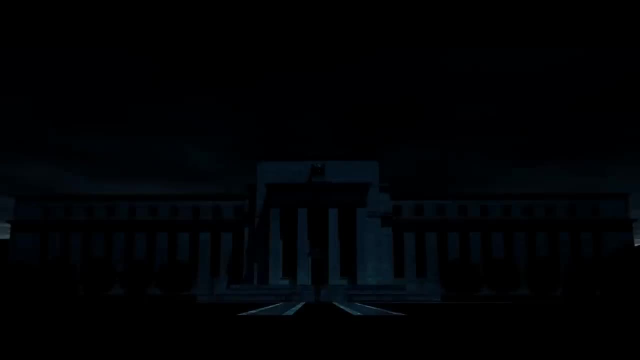 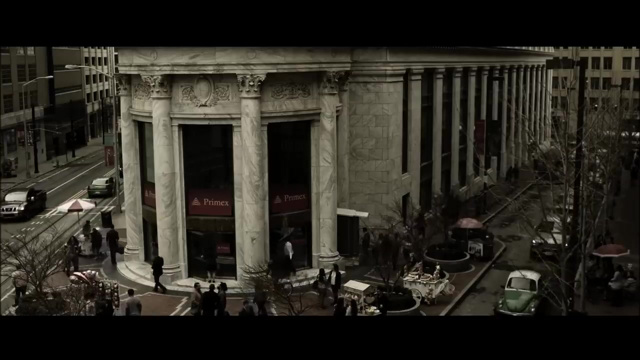 directly to the established value of gold. So in a country like the United States, one dollar was pegged at exactly 1, 50th an ounce of gold. This system was set up that in such a way, ideally, it would provide a stable monetary environment around the world. And it did for a while. but, as with all natural resources, the supply of gold was not as fixed as we originally thought. As a result, countries began dropping it as a means to measure the value of the money. In 1971, US President Richard Nixon officially severed the convertibility. 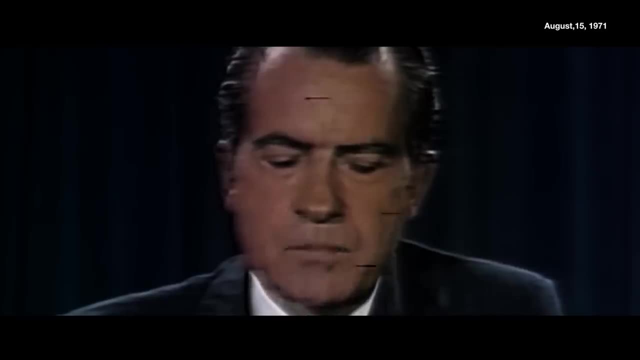 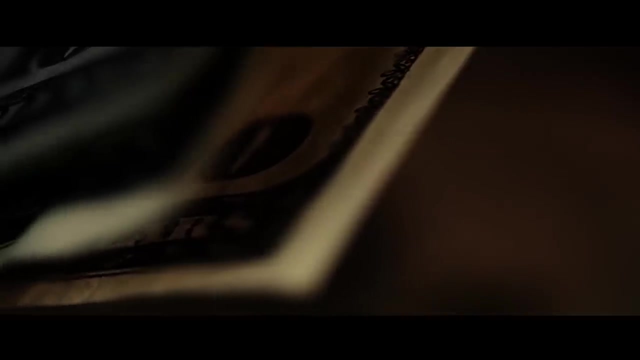 between dollars and gold. I have directed Secretary Connolly to suspend temporary the convertibility of the dollar into gold or other reserve assets. By that time the US dollar was seen as the global standard currency. so once the dollar was no longer dictated by the value of gold, pretty much nothing else was. 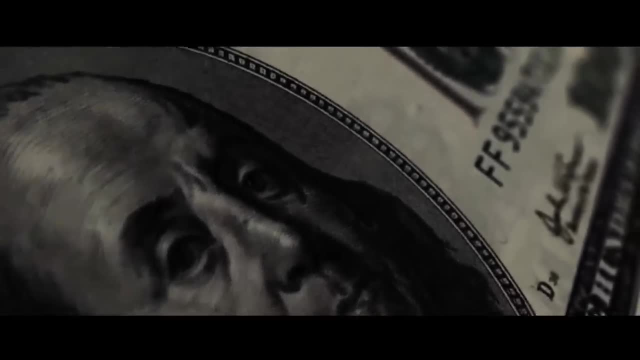 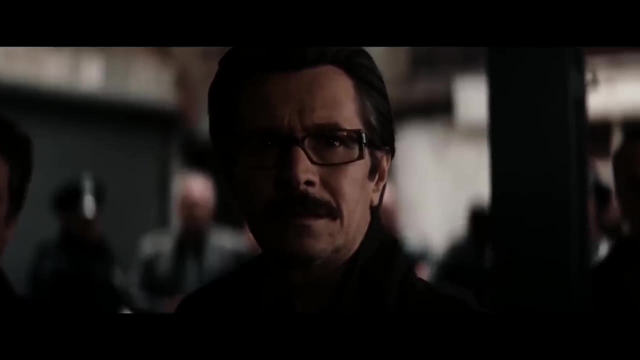 If the value of the dollar is no longer determined by the value of gold, what exactly makes one dollar worth one dollar? Well, instead of a commodity-backed system like the gold standard, we now have something called fiat currency, which has no intrinsic value. 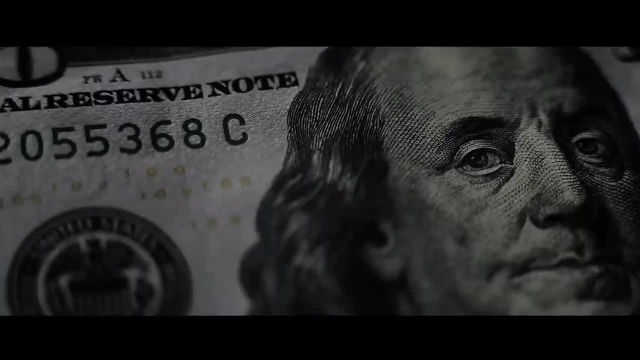 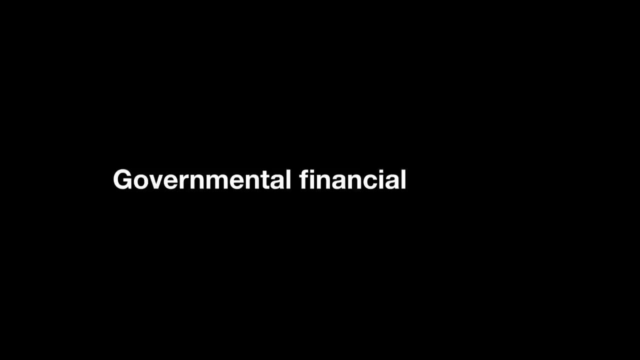 and is instead backed by a currency-backed system which is called fiat currency. What gives today's dollar its value is the economic supply and demand in the United States, and who controls that Governmental financial systems? In the case of the United States, it has the treasury and the US Mint in charge of printing. 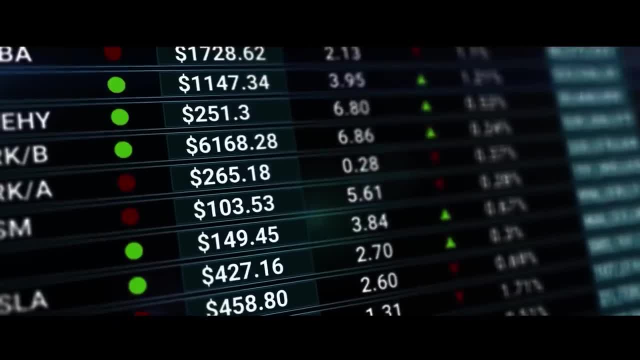 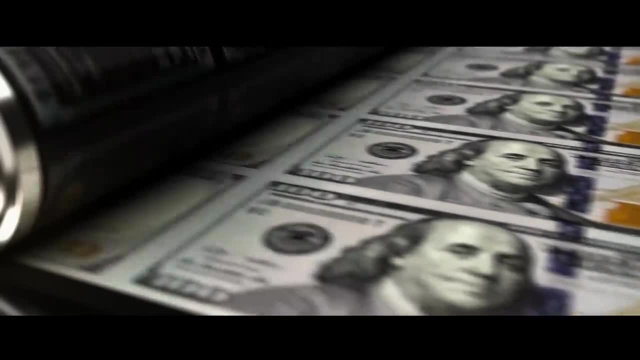 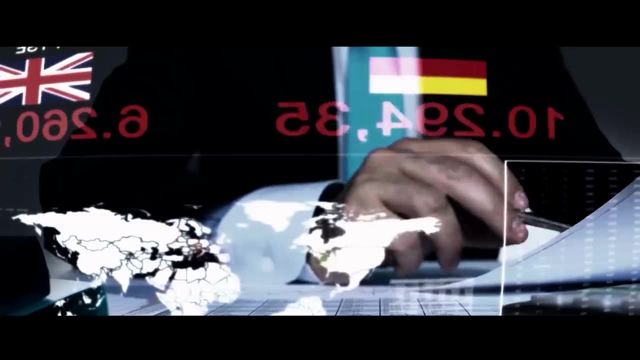 its money. But as we can see in the growing number of digital businesses and iPads in place of cash registers, money printing is a dying business. So if a government isn't literally printing money, how exactly does cash come into circulation? The vast majority of money exists only as numbers on a computer. 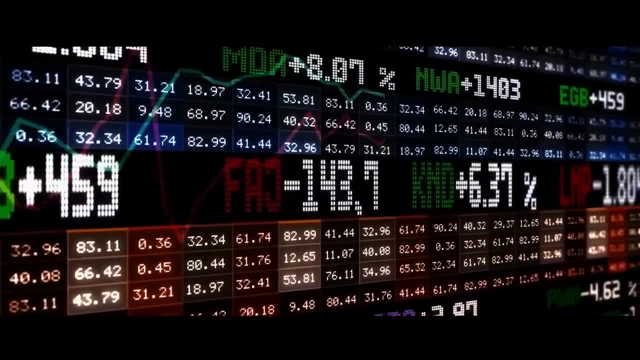 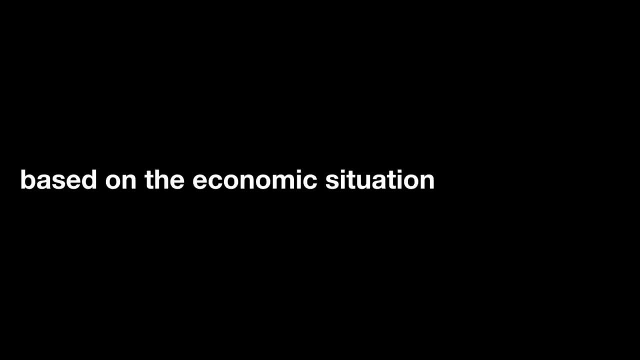 incredible amounts of money digitally credited to commercial banks by a country's central bank. This central bank controls how much money it deposits into the commercial banks based on the economic situation of the country. During the earlier stages of the pandemic in the US, some of that money was sent directly. 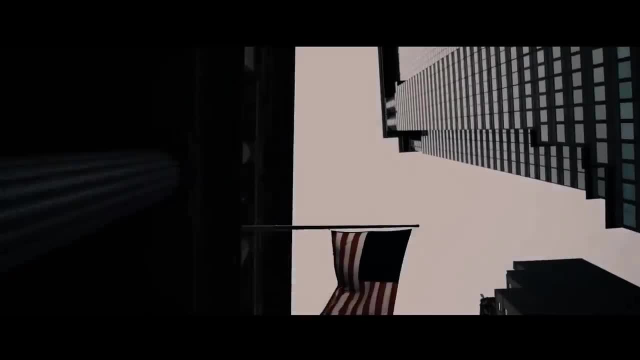 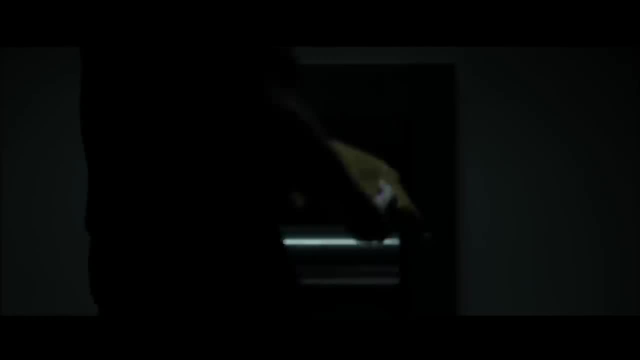 to bank accounts in the form of stimulus checks, But that's an extreme case and most of the time that's not how the money ends up with us. Here's how it usually works: A central bank sends money to banks and credit unions nationwide, and they in turn distribute. 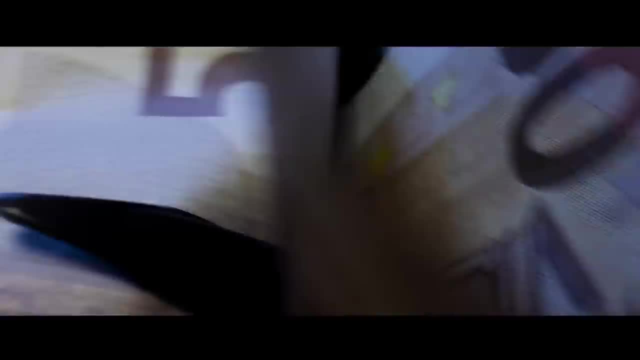 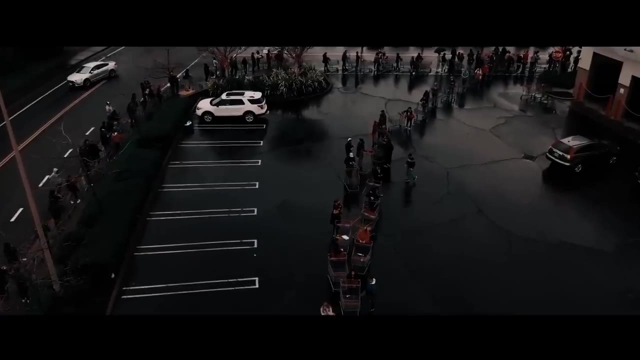 that money into the economy by lending it to their customers. Which brings us to the topic of debt. Around 80% of Americans are in some kind of debt, yet many people don't know what exactly debt is and how its moving parts work. What they do know, and what is backed by several studies, 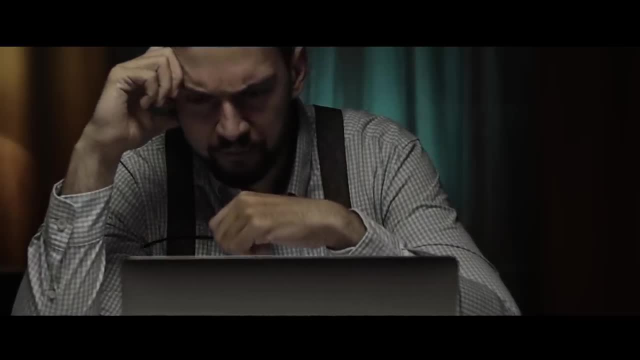 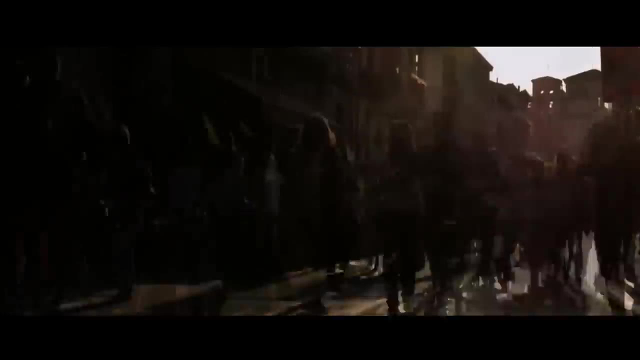 is that even the idea of paying off debt can be a severe emotional strain. No one wants to owe anyone anything, but with the cost of living vastly outpacing the money we earn for a living. Loans are the necessity everyone hates, yet most can't live without. 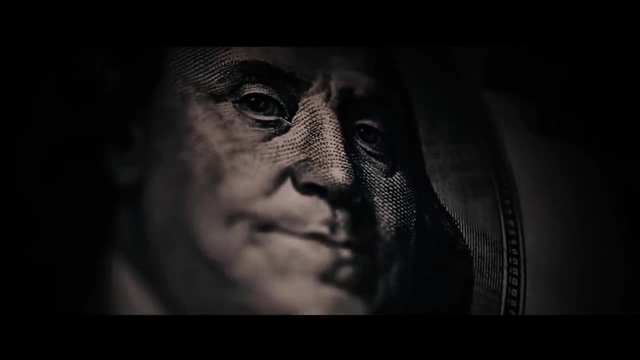 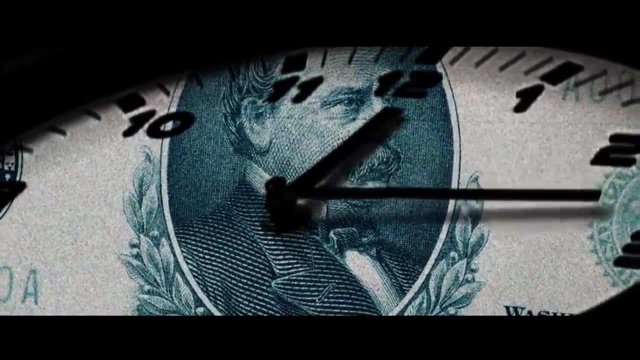 You get a loan to purchase your car, start your small business, go to college or buy a house. Very few people can afford a house with the money in their bank accounts, yet all of us need a roof over our heads, So some people choose to rent. 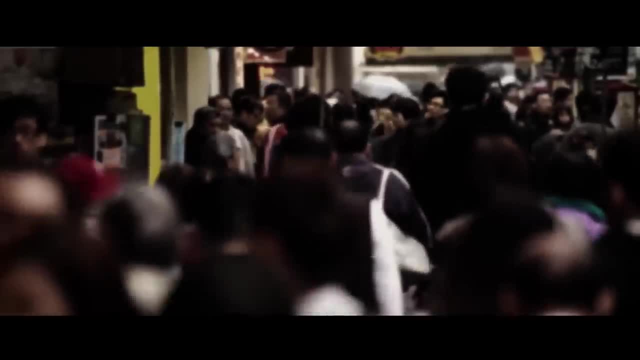 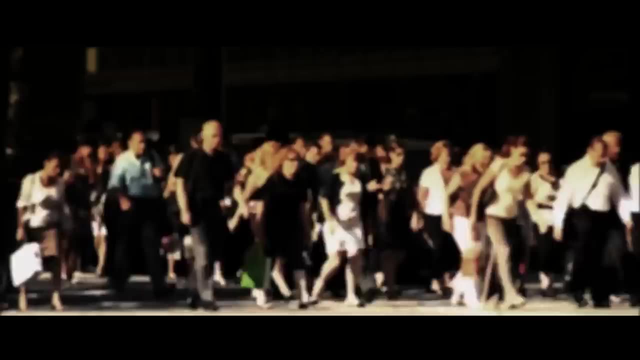 while others decide to take out a loan from the bank in the form of a mortgage. But banks aren't charity organizations. they're built to make a profit, and the way they do that is through interest. Interest is the amount you, the borrower, pay to use the money a bank or financial institution has loaned you. 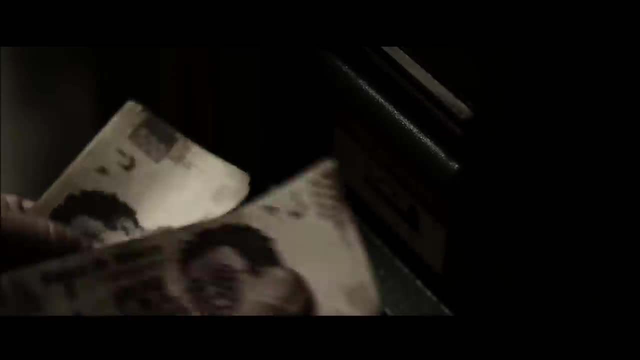 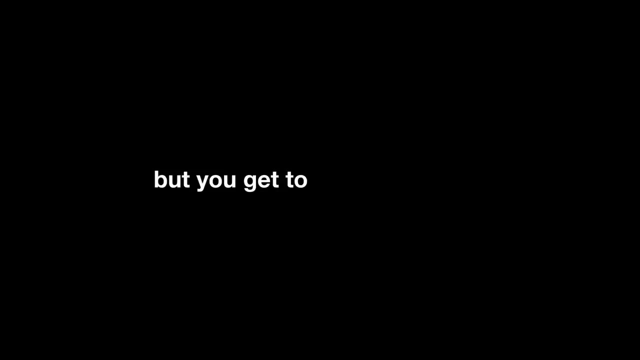 Think of it like the rent you pay on your apartment every month. You don't own the apartment, but you get to use it for a fee. In the same way, you don't own the money you use to purchase your house, but you get to use it for a fee. And this: buy now, pay later. model. 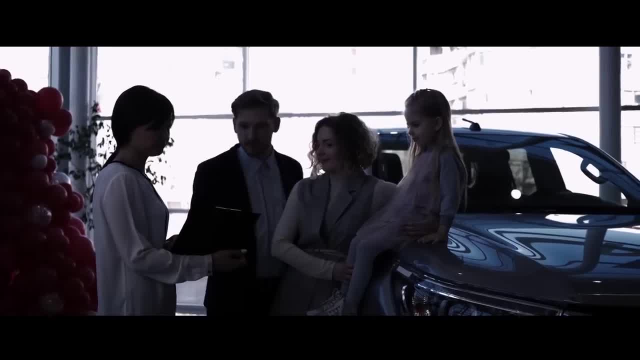 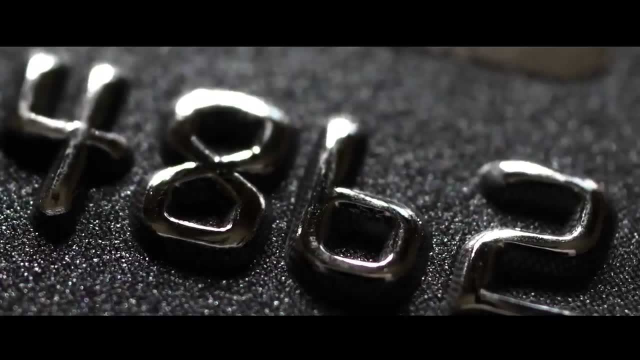 does not only exist for big purchases like a house and college. It has permeated our entire society so much that most things we purchase now exist on this model, Especially since the creation of the credit card. Don't have enough cash for that new couch? Put it on your credit card. Want to get. 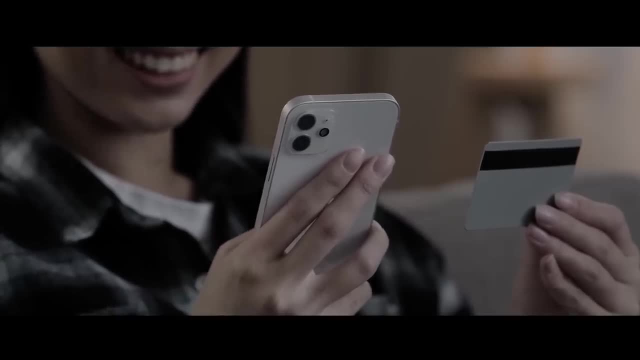 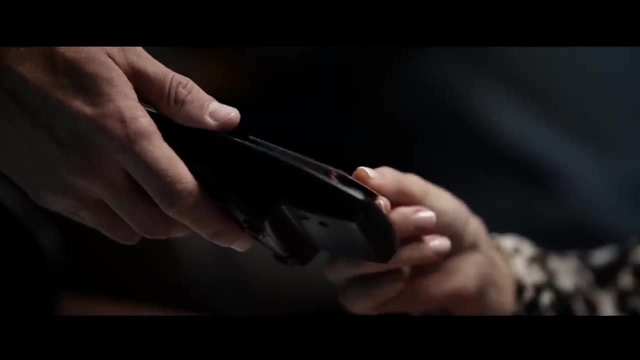 that new iPhone Pay a monthly fee to your internet service provider. Heck, even consoles like the Xbox follow the same model. We now use credit to pay for even small things like a sandwich, a new pair of pants or food for our dogs. If we pay our balances on time for those. 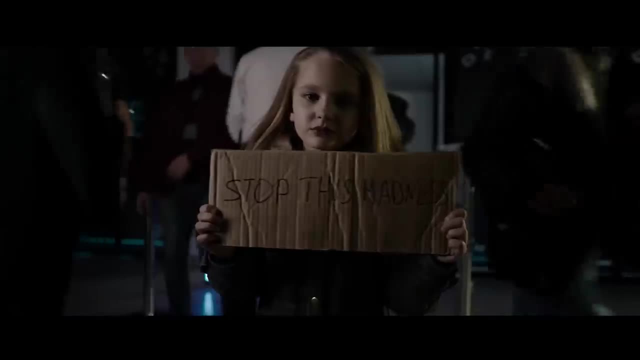 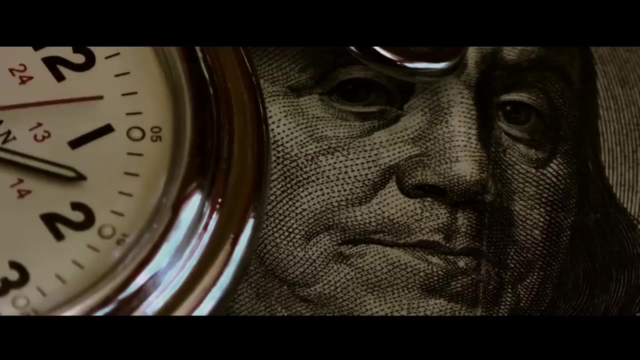 purchases, we can avoid the interest rates that credit card companies charge and we'll be fine. But for a lot of us, especially in hard times, we tend to build interest on our cards, which can quickly lead to a pretty bad spot financially. Credit cards can help provide. 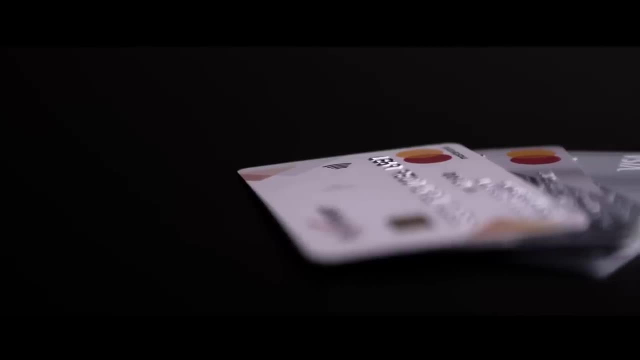 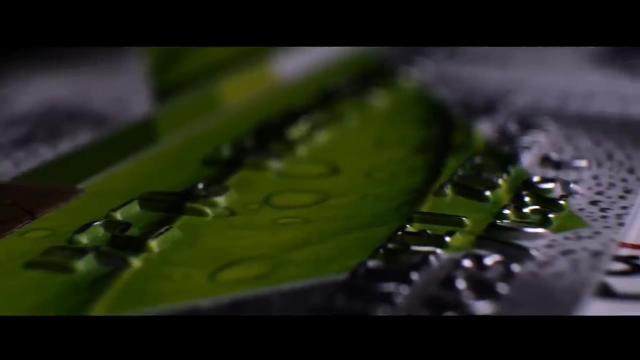 a financial buffer in a bind if needed. but they also come with an element of risk, So are they worth it? There's some mixed feelings about this. Some people think that using credit cards is a surefire way to send yourself straight into sinking debt, But others see frequent credit. 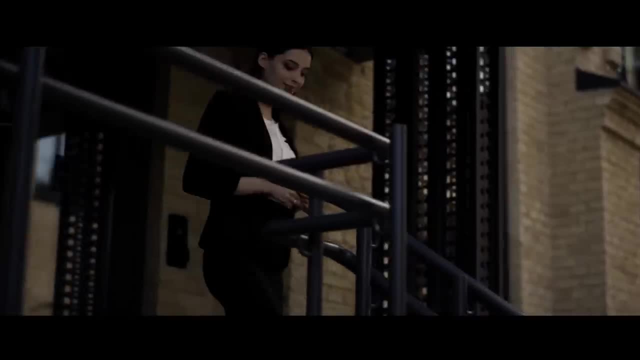 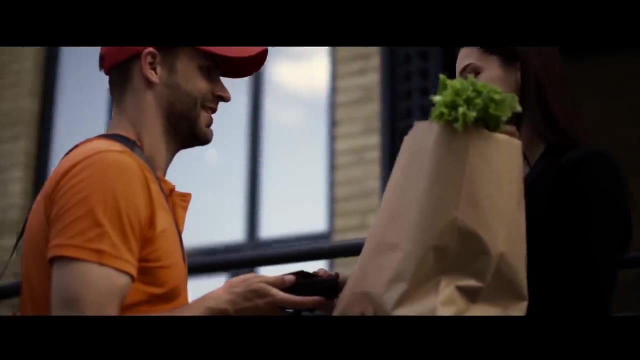 card use as a way to build good credit, which, if you've ever leased an apartment or bought a car, is an important part of daily life these days. Whichever side of the fence you're on, one thing we can all agree on is that you need to be careful when using credit cards so that you 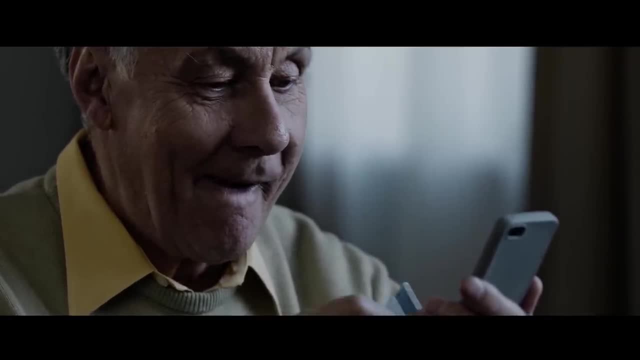 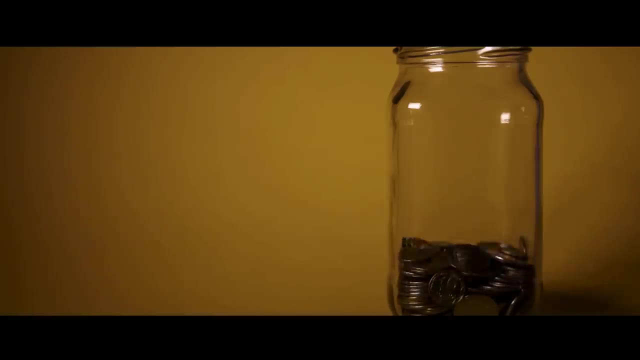 don't overspend and dig yourself into much deeper debt than is necessary. By being wise with your credit savings and increasing your income, you can have enough disposable income to finally do with your money what every financially stable person suggests: Invest. Investing basically means: 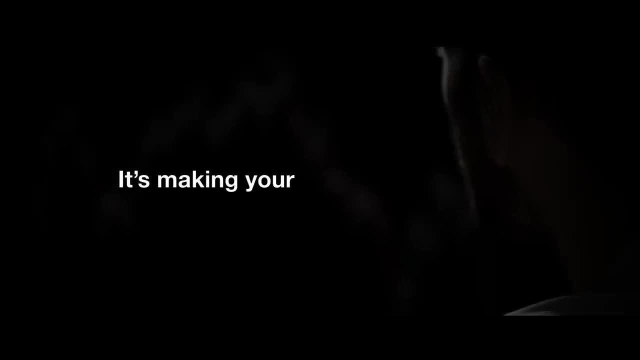 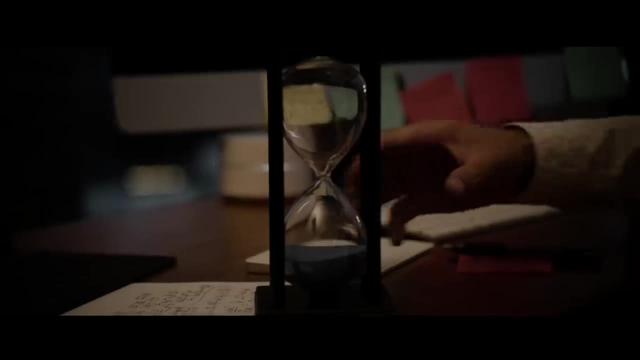 committing your money to something to earn a financial return, It's making your money work for you. One mantra in the investing world is: the greater the risk, the greater the reward. Investments like bonds are safer but offer lower returns, while investing in individual stocks can. 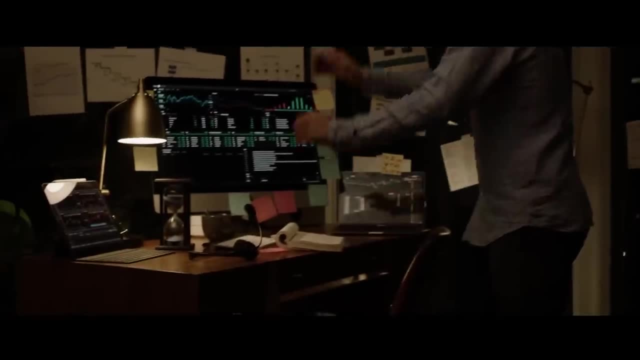 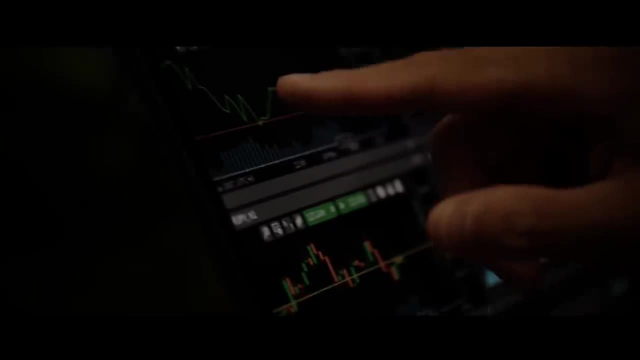 provide incredibly high returns but are also extremely risky. And let's not even get started on cryptocurrency. We'll need an entire video to go over investing properly. but in the end, if we get the opportunity to do so, our goal is to build our wealth, To increase how much we're worth. 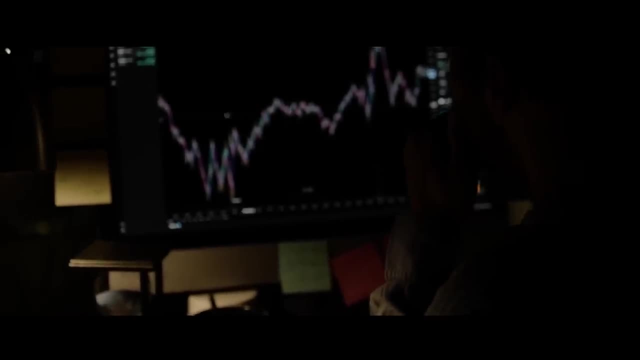 and that's the entire point of money: to show how much something or someone is worth. How much is a carefree retirement to you? Let me know in the comments below, And if you want to see more of my videos like this one, be sure to subscribe to my channel and hit the bell so you don't miss out on. 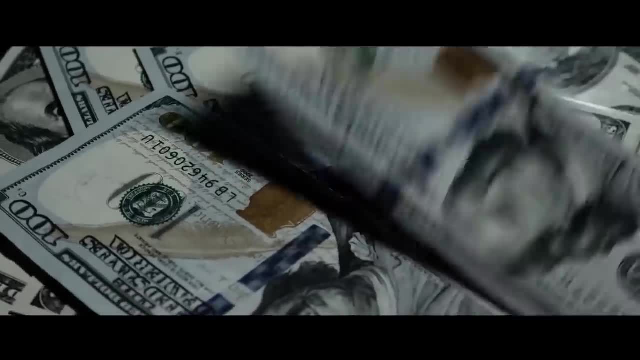 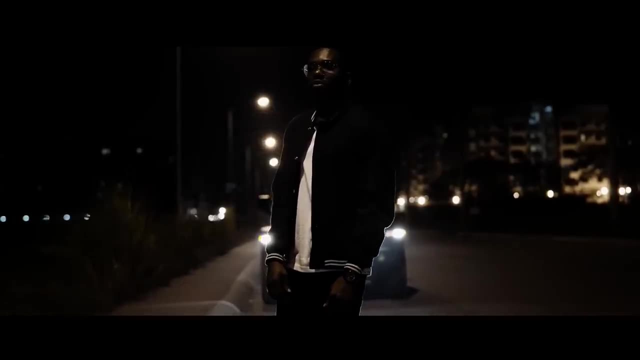 any future videos That will inform how much money you put away in your retirement account? What about a car? We might splurge on a luxury vehicle because it's worth it to us to enjoy the extra comfort and social status. The byproduct of this is that, as a society we've become, 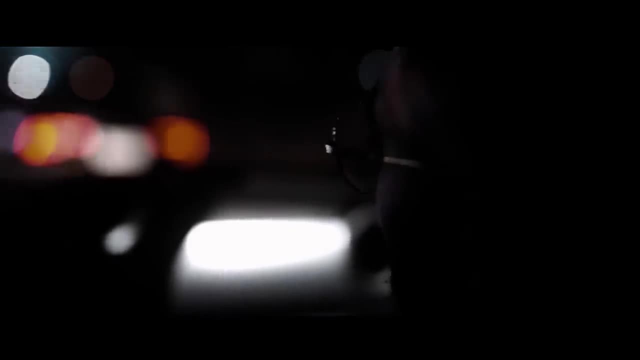 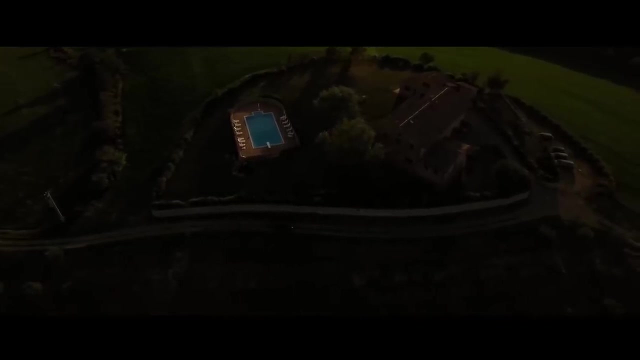 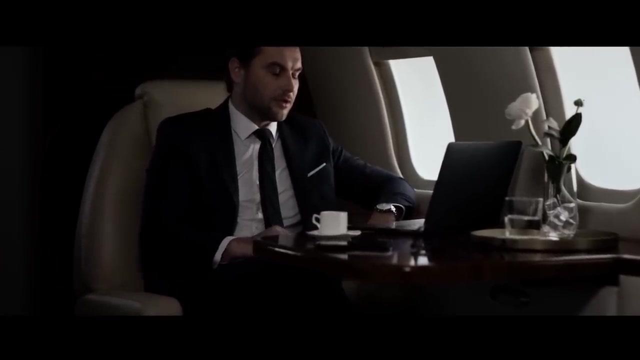 obsessed with the idea of worth, from material goods and worldly possessions to personal worth and even that of others. Publications like Forbes and Bloomberg publish wealthy individuals' net worths, assigning a number to someone's success To create these lists. dozens of reporters track down millionaires and billionaires all across the world, collect their personal.